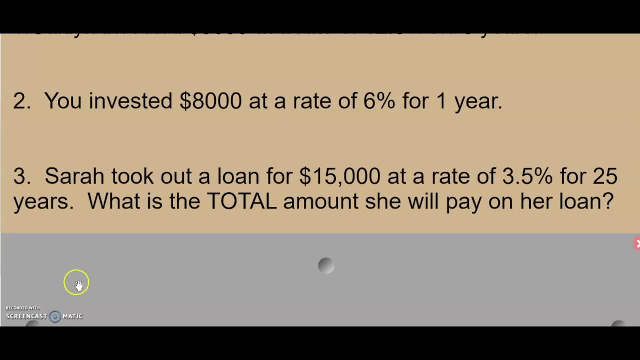 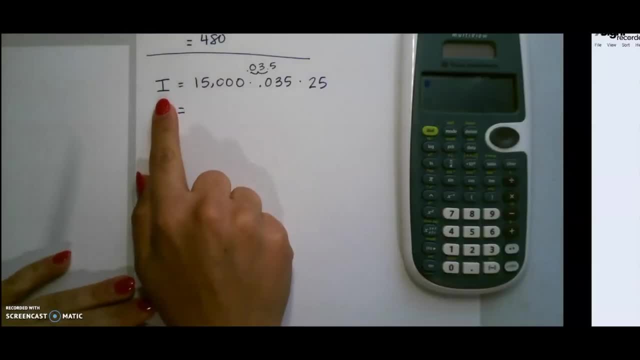 What is the total amount she will pay on her loan. Total is capitalized here because we're going to do something a little bit different. First, we're going to find the interest, just like we have on the two previous problems. $15,000 is our principal amount. 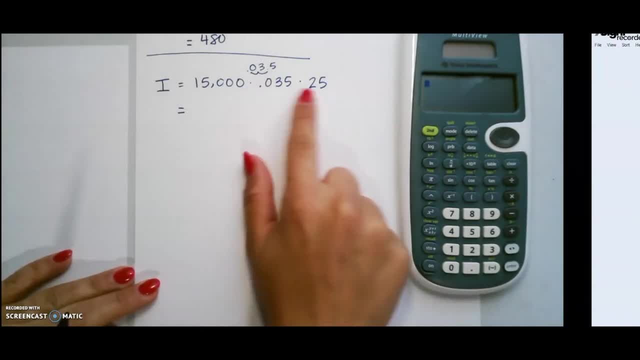 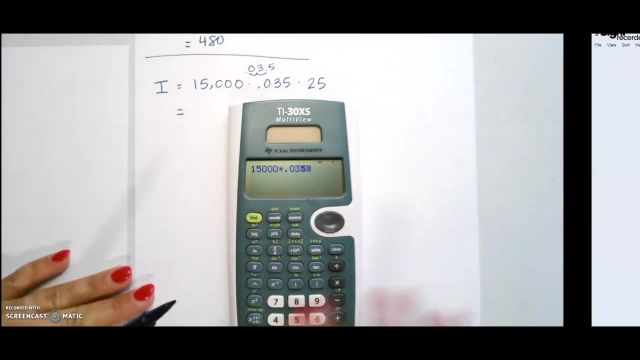 3.5% was our principal amount. 3.5% was our principal amount, So we changed it to a decimal And our time was 25 years. So we plug that into our calculator And this gives us our interest. 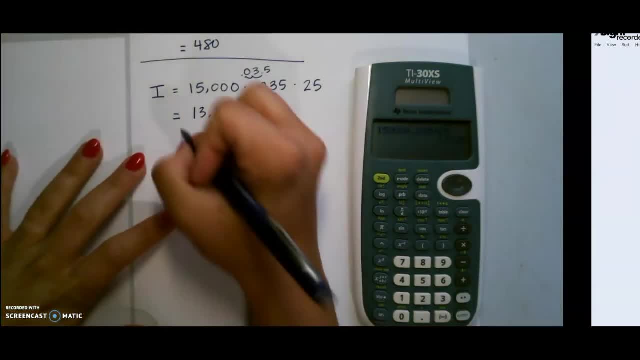 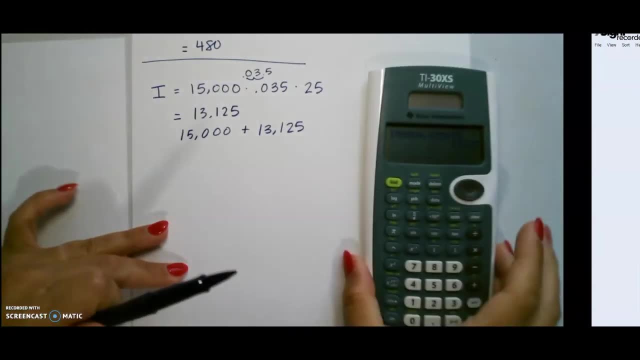 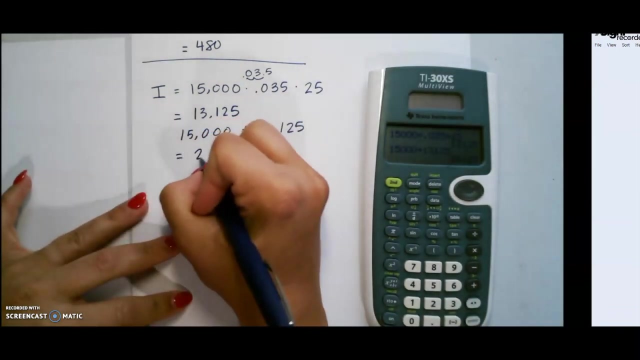 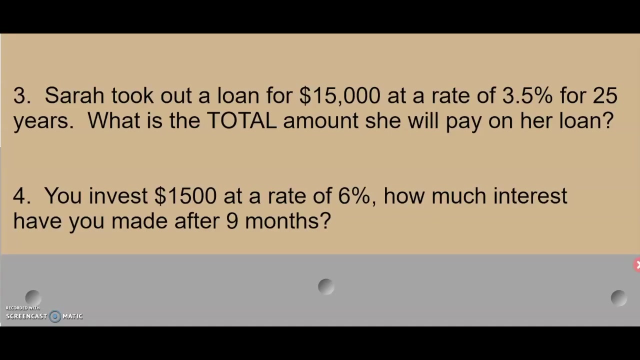 Since it asked us for the total amount that they will pay on the loan. we would then add our principal amount plus our interest to get our total. So we can simply add this To get a total payment of $28,125.. For our last example, you invest $1,500 at a rate of 6%. 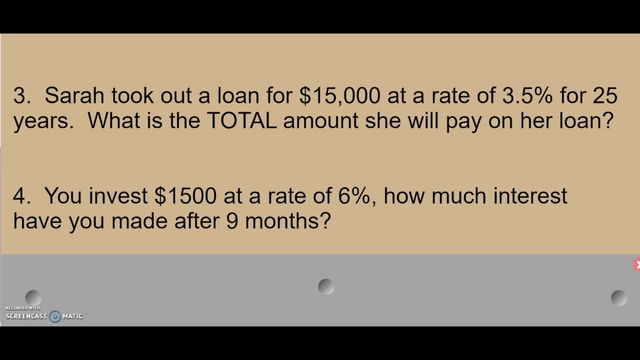 How much interest have you made after 9 months? I want to show you this example because it discusses 9 months. We look at time in terms of years for these, So we need to figure out how to change 9 months into terms of years. 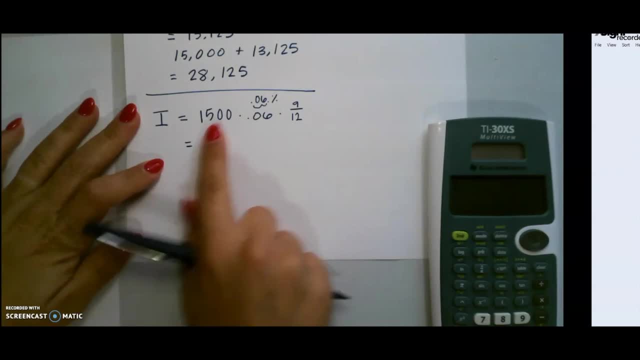 So for this one, $1,500 is our principal amount, So we plug that into our calculator. 6% as a decimal is .06.. And here we have a fraction. So since we were talking about 9 months, there are 12 months total in the year. 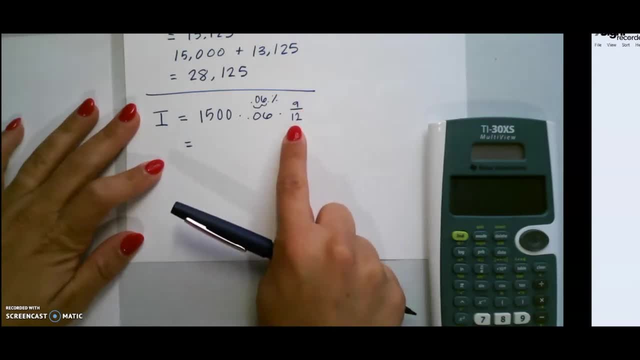 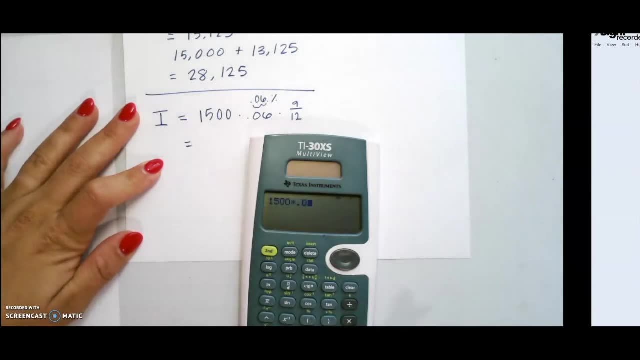 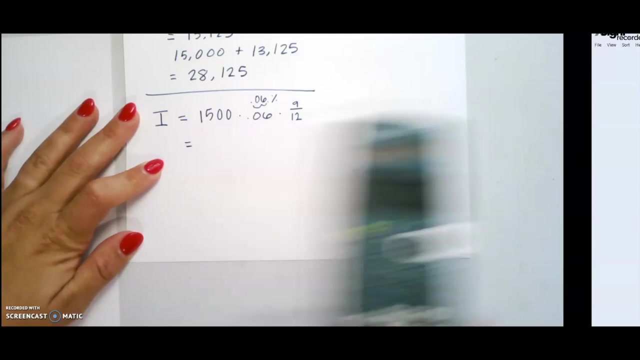 So we just simply put 9 over 12 to multiply that for our terms of years. So then we plug this into our calculator And if you have a multi-view calculator, you can use the fraction button And that will give us 67.3%. 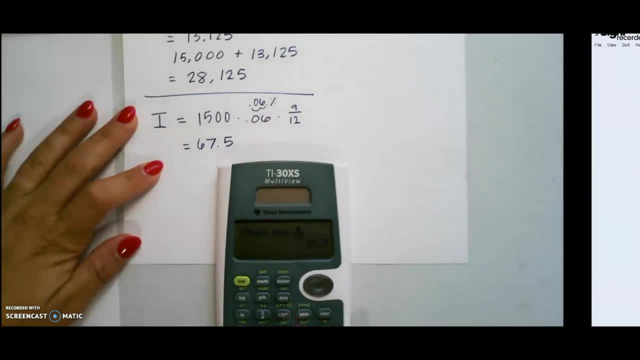 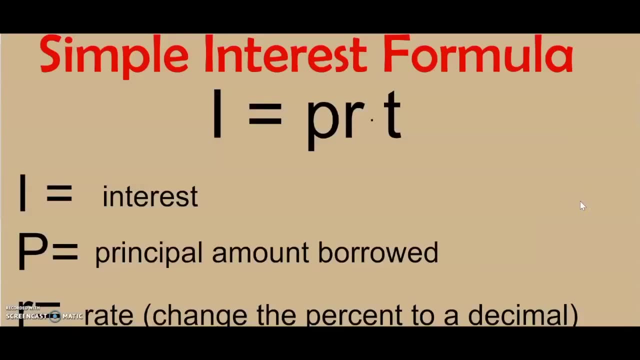 If you do not have the multi-view calculator, you can change this to a decimal And then use the multiplication method As a final review. to find simple interest, use the formula I equals PRT, In which the I stands for interest, the P stands for the principal amount borrowed. 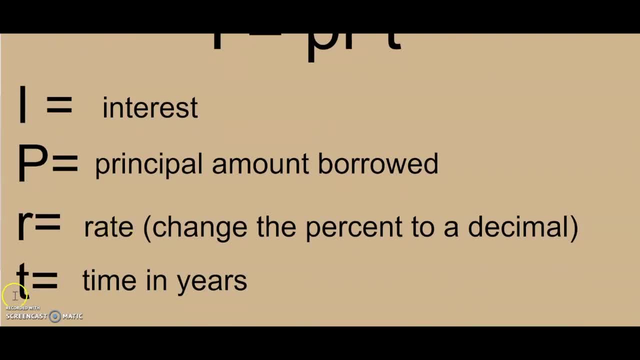 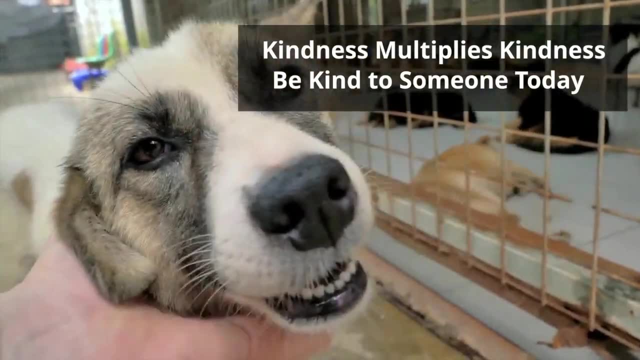 the R is the rate and the T is time in years. Thank you for watching this video. If you have any questions, please feel free to ask them in the comments.